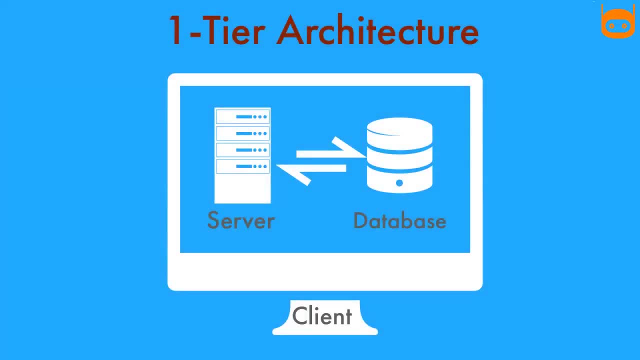 architecture- one tire architecture. one tire architecture is that where the client server and database all reside on the same machine. anytime you install a db in your system and access it to practice sql queries, it is one tire architecture. for example, while creating a web application by java programming language, we have installed apache server and mysql database within. 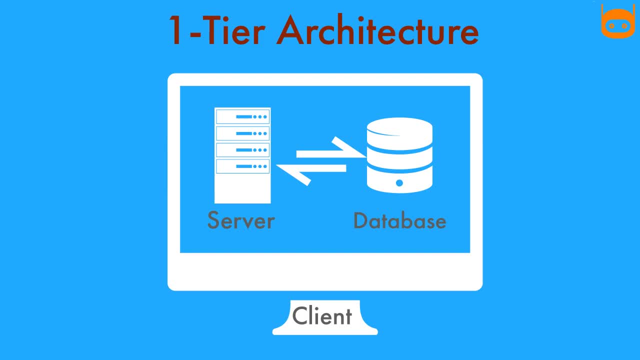 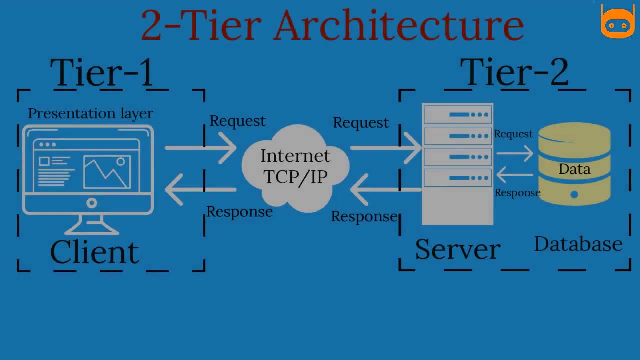 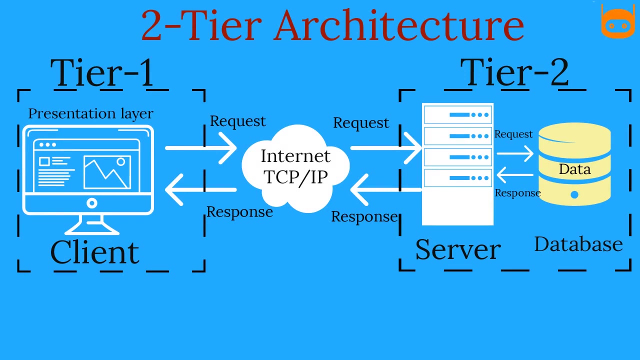 our machine to run our web application. we don't need extra physical server and database outside our computer. two tire architecture. the two tire architecture is that where presentation layer runs on a client and data is stored on a server. in this architecture, a client request for data or resources. 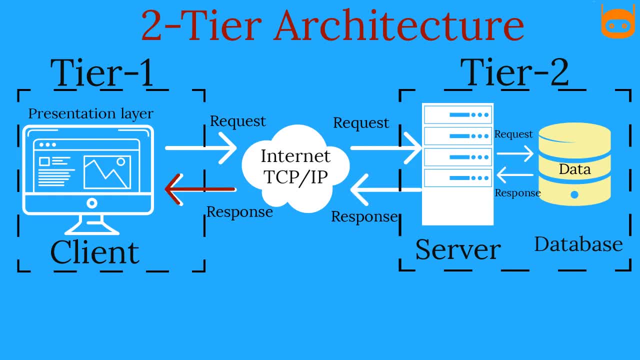 to server and server process that request entire one. our clint resides in entire two server and database or occur. these both tire are communicate with each other through the internet or any network. this structure is quite easy to maintain and modify. the communication between the client and server in the form of request response and messages transfer is quite fast. the major drawback: 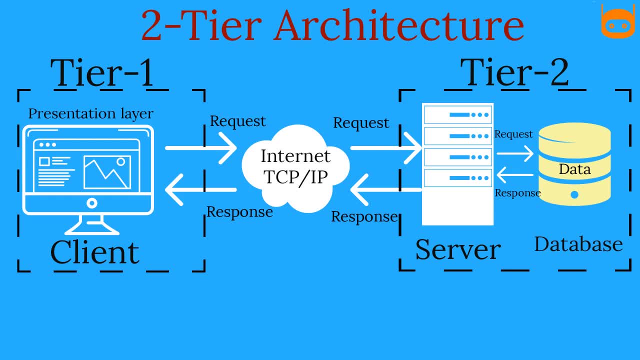 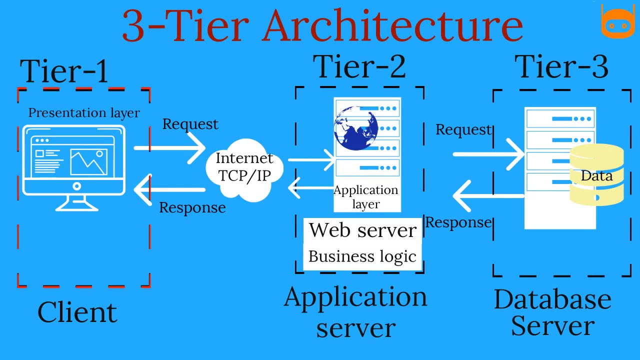 of this structure is: if the client nodes are increased beyond capacity in the structure, then the server is not able to handle the request overflow and performance of the system degrades. three tire architecture. the three tire architecture has three layers, namely client application and data layer. the client layer is the one that requests the information. in this case it could be the guay. 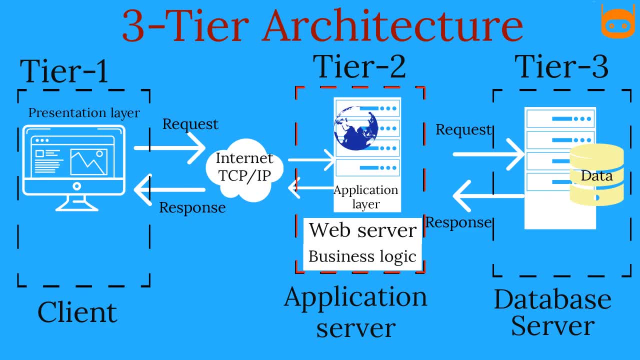 web interface, etc. the application layer acts as an interface between the client and data layer. it helps in communication and also provides security. the data layer is the one that actually contains the required data. this architecture contains an application between the user and the DBMS, which is responsible for communicating the user's request to the DBMS. 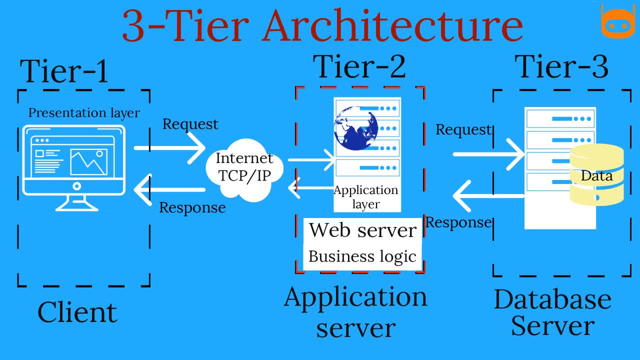 system and send the response from the DBMS to the user. The application layer, also called business logic layer, that processes functional logic constraint and rules before passing data to the user are down to the DBMS. Three-tire architecture is the most popular DBMS architecture.